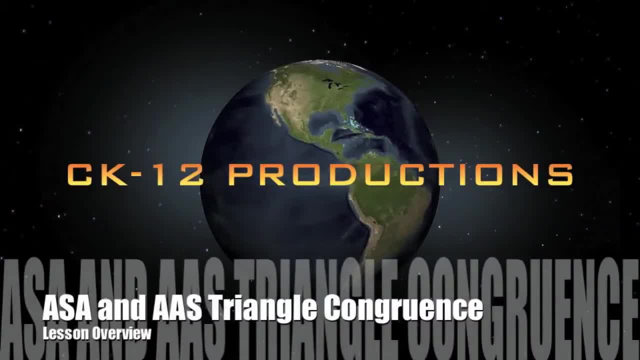 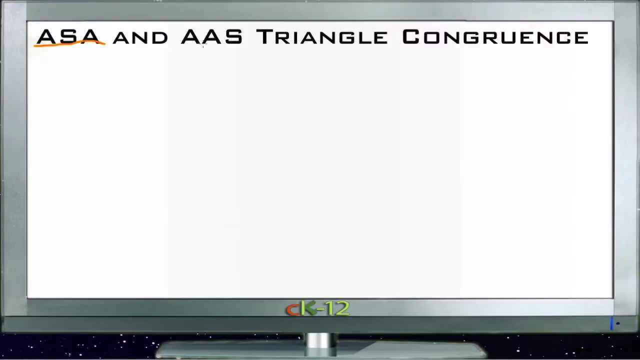 All right, let's talk about angle-side-angle and angle-angle-side triangle congruence. Again, order is very important when we're discussing these rules. These are again more shortcuts for finding out whether two triangles are congruent in all ways. 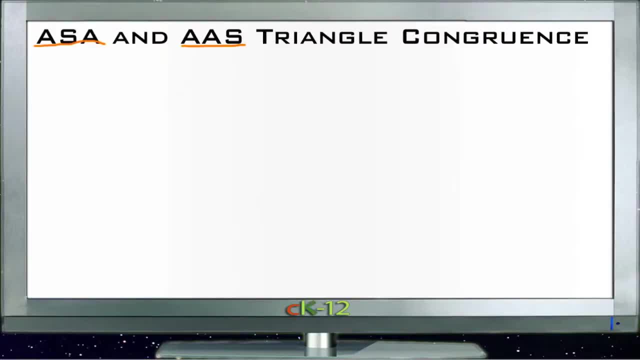 without having to worry about finding all the sides and all the angles. The first one we're going to talk about here is the angle-side-angle. So this one is ASA, And angle-side-angle tells us that if we know that the angle of two triangles is the same, 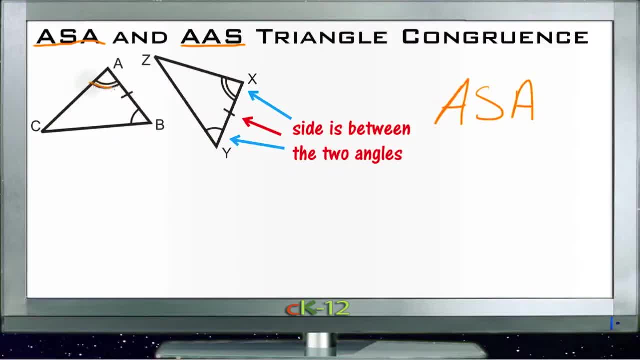 Let me draw on top of that so we can see better. So if we have one angle, this one is a double hash mark and it's corresponding to the double hash mark over here And then in between it and another angle, that is also the same. 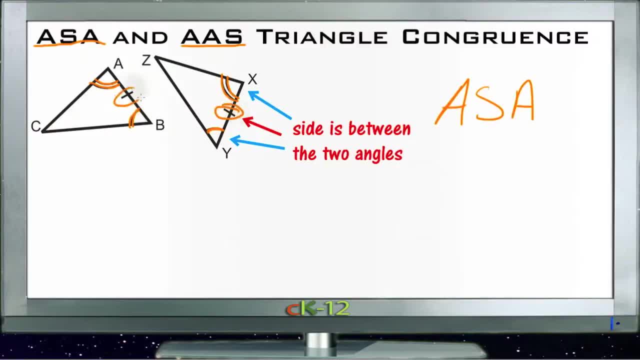 we have a side that is the same, then we know that those two triangles are congruent. Now again, as I've kind of done before, we can sort of think about this logically a little bit. If you recognize that you have a set angle and a set length of a side, 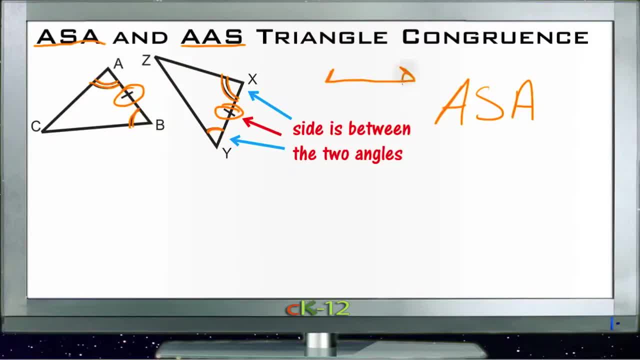 and another set angle right here. So if we assume that this angle here and this angle here are fixed and the length of this bottom side is fixed, then from that point it doesn't matter what I try and do with these other two sides up here. 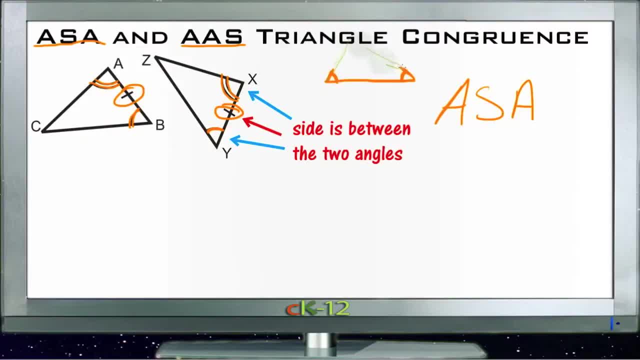 They're only going to meet in one place. They can't meet anywhere other than that one place, no matter how long I make them. I mean, if I make them too long, they may cross over each other like so, But they're still going to meet in that one location, no matter what I do with the lengths of those sides. 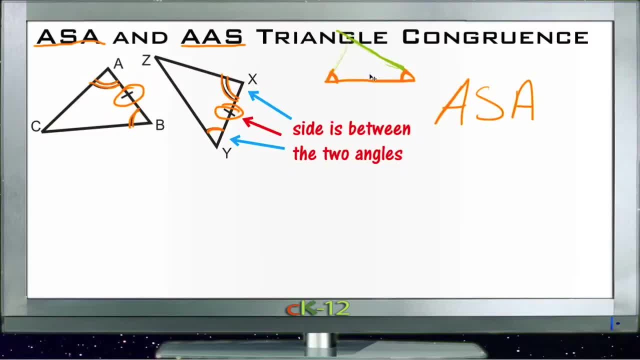 So we can see that there's only one triangle that can be made with a fixed set of angles and the side in between them of a fixed length. So, angle-side-angle- Angle-side-angle tells us that we can identify two congruent triangles just with that information.